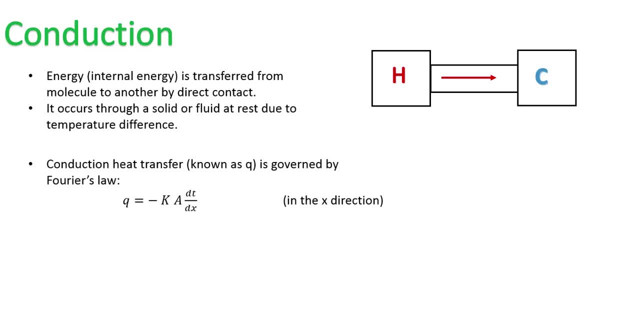 Conduction, heat transfer, which is denoted by Q, is governed by Fourier's law. Its equation is: Q equal minus K, A del T by del x, Where K is the material's conductivity, del T is the temperature gradient and area is. A is the area of which the surface is perpendicular to the direction of the. 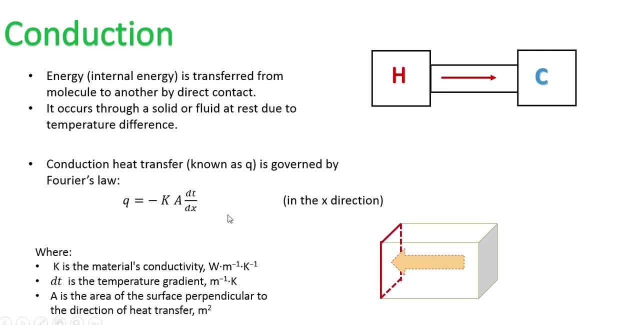 heat. Here is the area. Now, the negative sign in this formula here is because the temperature final should be less than the temperature initial in order for the heat to move. But it also can be written in this form in order to get rid from the minus sign: 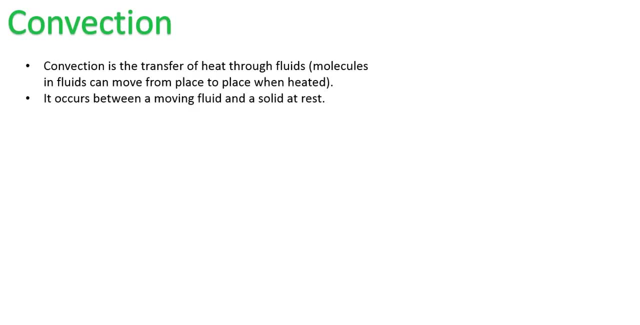 Second method is convection. Convection is a method by which heat transfers through movement of the the medium. for example, in fluid, molecules can move freely from place to another, especially when heated. it also occurs between a moving fluid and a solid at rest. let's take this example. suppose that we have a hot object inside. 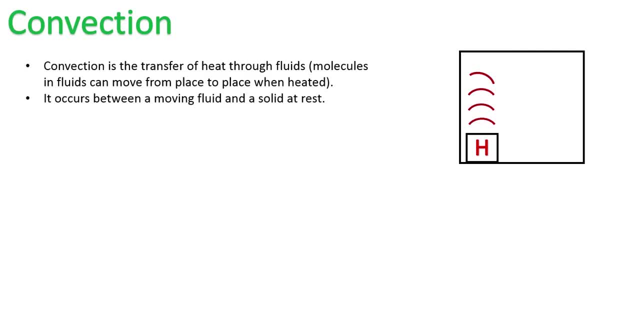 a room. this hot object will heat the air up around the air, will expand and heat the port above it, and so the heat travels with air. now, the reason of why hot air rises is because when air becomes hot, it expands and molecules will become less closer to each other's, which decrease its weight. thus cold air. 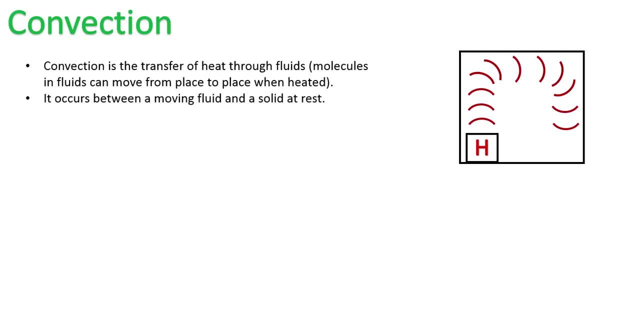 which is denser, pushes hot air upward. convection-heated transfer, which is known as Q, is a heat transfer, which is known as Q, is governed by Newton's law. its formula is H, A, T, S minus C surrounding, where H is the convection coefficient. heated transfer- we'll talk about it later. 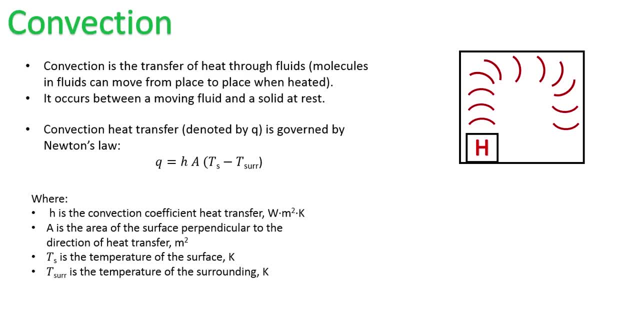 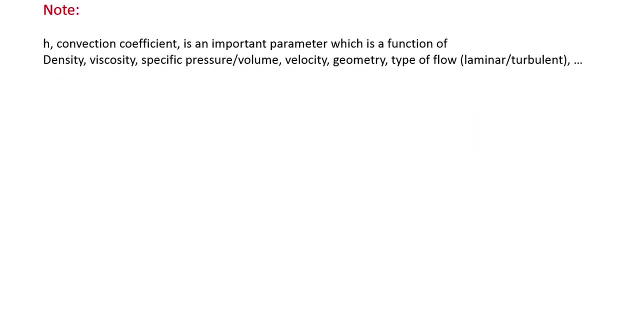 A is the area. T is the temperature of the surrounding or the surface. in our case, temperature of the surrounding is a temperature of the room. temperature of the surface is the temperature of the hot body. here I want to highlight on the convection coefficient H, which is very 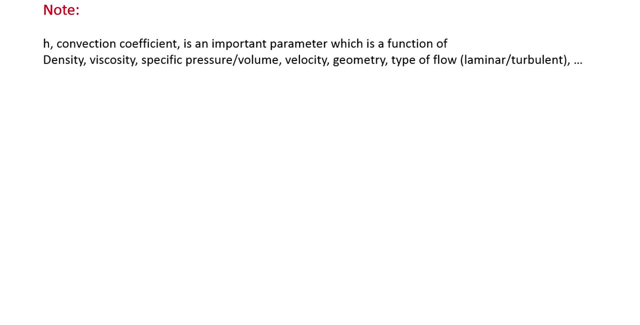 important parameter and there are many methods to calculate it. convection coefficient H is a function of density, viscosity, CP, CV, velocity, geometry, type of flow, etc. there are two types of convection. first one is a free or natural. the fluid motion here is natural, which is caused by natural means, and the 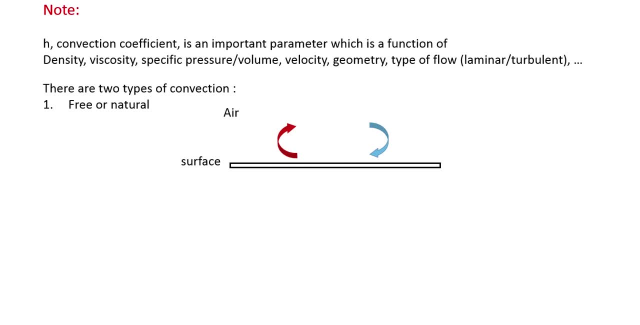 such as buoyancy. Buoyancy is the rise of warm fluid and fall of the cold fluid. We mentioned this before. The first convection is the fluid here. fluid motion here is generated by an external source such as pump, fan, suction device and many others. 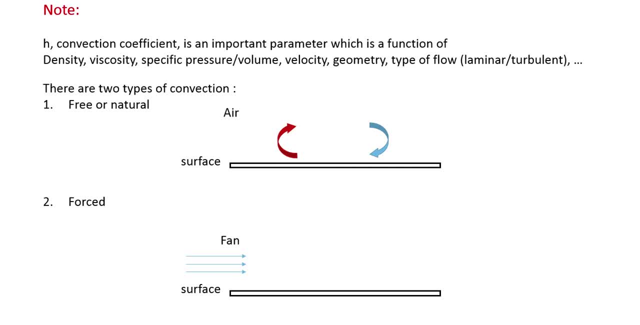 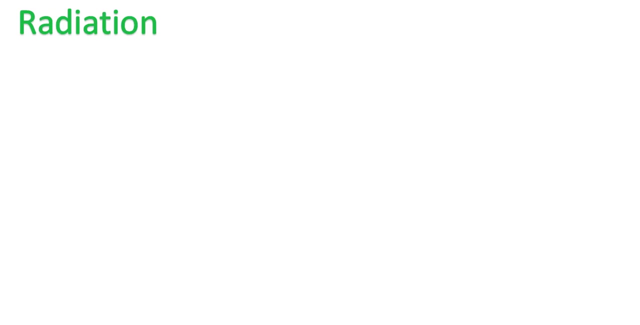 If we want to compare both types or methods here, it's obviously clear that forced convection, heat transfer and forced convection is higher than the heat transfer of the free convection. Now the third mechanism is radiation. It doesn't need a medium at all. 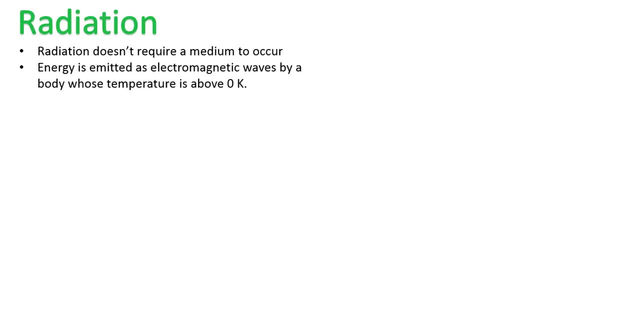 where energy is emitted as electromagnetic waves by a body whose temperature is above zero Kelvin. When heat radiates, it goes in all directions. Stevens Boltzmann indicates that thermal radiation flux is equal to E minus alpha G, where G is the radiation incident on object from the surrounding, E is the emissive power of the object. 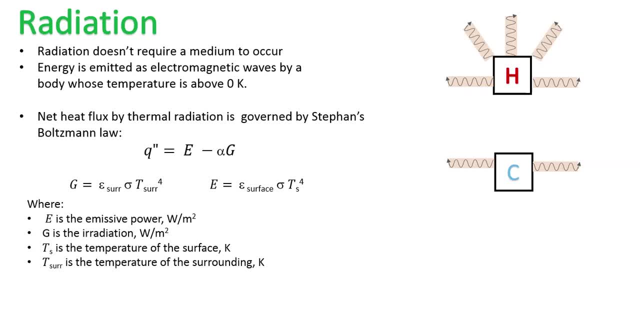 Epsilon is the emissivity of the surrounding or the surface, Sigma is Stevens Boltzmann constant and T is the temperature. Now, the emissivity. epsilon is a dimensionless constant that varies between 0 and 1 if it indicates the ability of the body to emit energy. If Epsilon is 0, then the body is a perfect reflector. 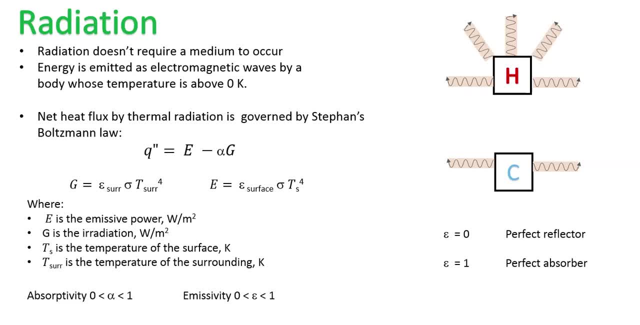 If Epsilon is weak, then the body is a perfect reflector. if epsilon is one, then the body is a perfect absorber. usually surrounding is considered as a perfect body, although perfect bodies do not exist. similarly, absorptivity is a dimensionless constant that varies also between zero and one.